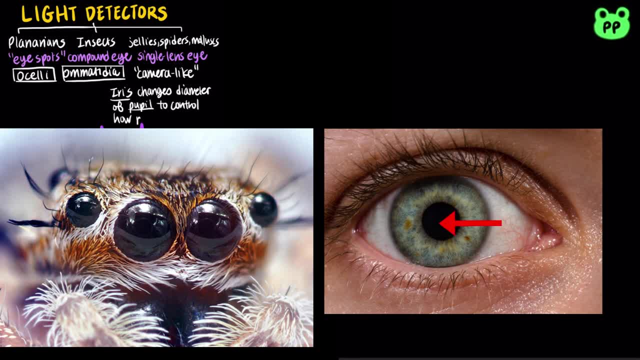 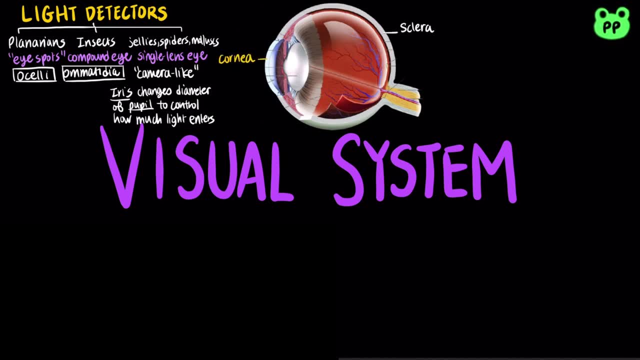 The iris changes the diameter of the pupil to control how much light enters. The main parts of a human eye include a white outer layer called sclera, which forms the transparent cornea. Beneath the sclera is the pigmented layer called choroid, which forms the 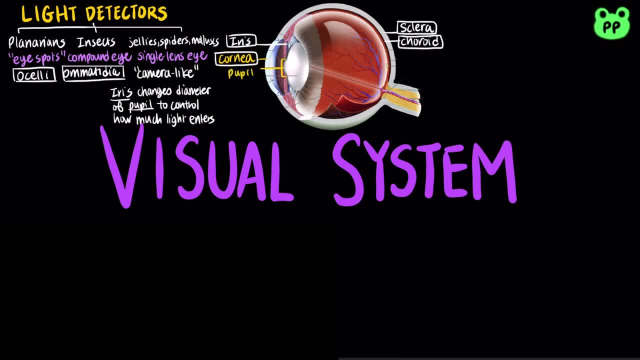 colored iris. The iris regulates the amount of light entering the pupil by changing size. The pupil is also a single-lens eye. The pupil is also a single-lens eye. The pupil is the hole in the center of the iris. The layer inside the choroid is the retina. 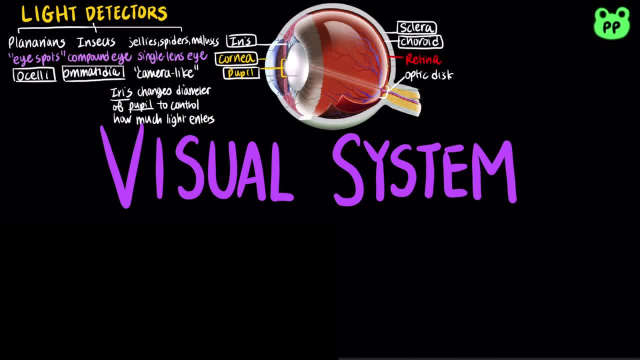 which contains photoreceptors. The optic disc is a blind spot in the retina where the optic nerve attaches to the eye. The lens is a transparent disc of protein that focuses light on the retina. The eye is divided into two cavities, separated by the lens and ciliary body, The anterior cavity. 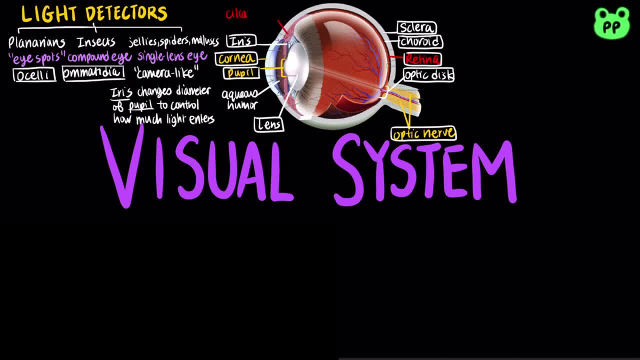 is filled with watery, aqueous humor, which is produced by the ciliary body, while the posterior body is filled with watery, aqueous humor, which is produced by the ciliary body, while the posterior cavity is filled with jelly-like vitreous humor. 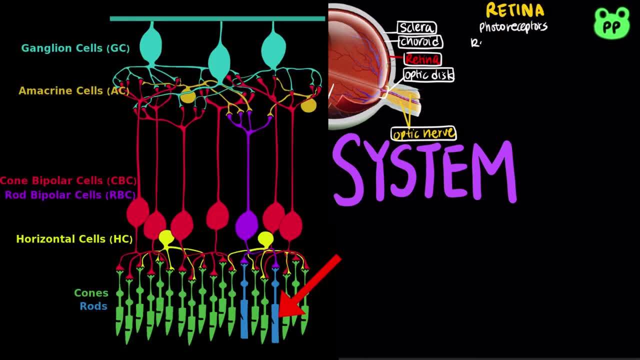 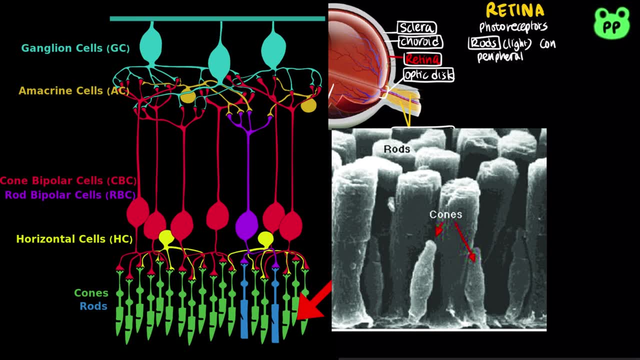 The human retina contains two types of photoreceptors. The rods are light-sensitive photoreceptors that are concentrated around the periphery of the retina, whereas the cones are photoreceptors that distinguish colors and are concentrated in the fovea, which is the center. 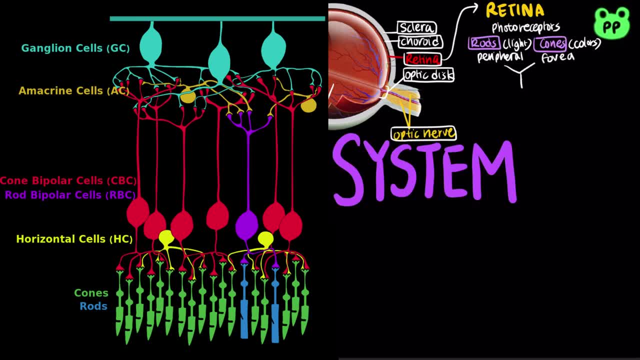 of the visual field. After the light reaches the photoreceptors, the bipolar cell receives information from several rods or cones, and each ganglion cell is concentrated around the periphery of the retina. The foot cell gathers input from several bipolar cells and relate the information to the optic nerve fibers. 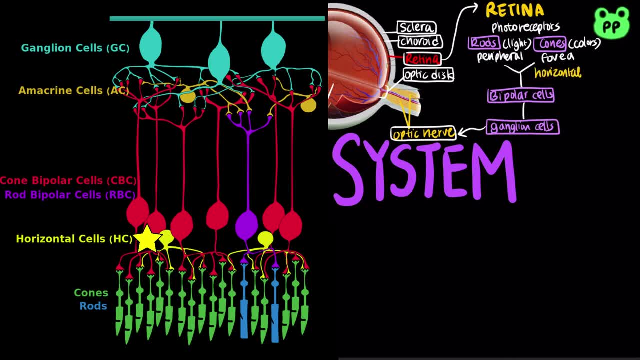 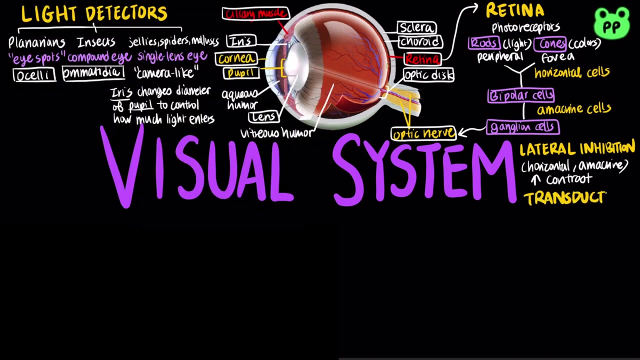 The horizontal Without big bone, 귀여winning つ horizontal benefiting, which consists of a light-absorbing molecule called retinol bonded to a protein called opsin. When light strikes the rhodopsin, it converts cis-retinol to trans-retinol. 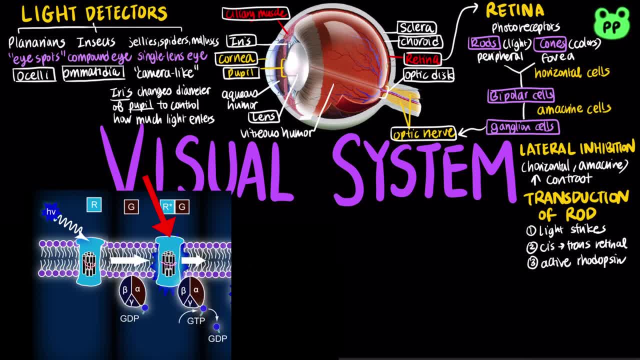 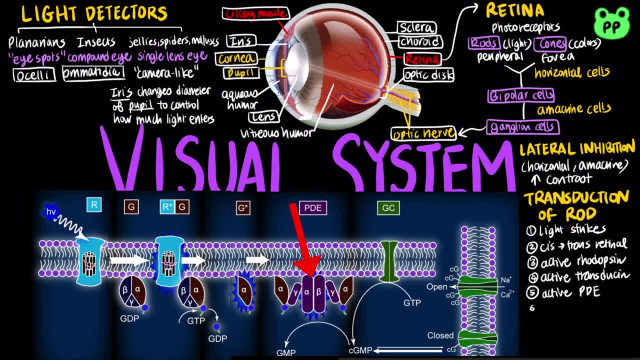 which activates rhodopsin. Active rhodopsin in turn activates G-protein called transducin. Transducin then activates the enzyme phosphodiesterase, which detaches cyclic GMP from sodium channels in the plasma membrane by hydrolyzing cyclic GMP to GMP. 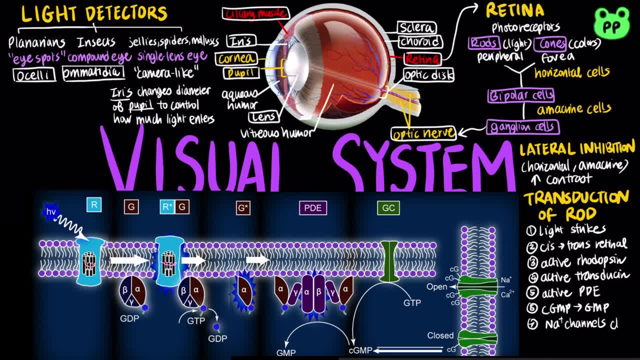 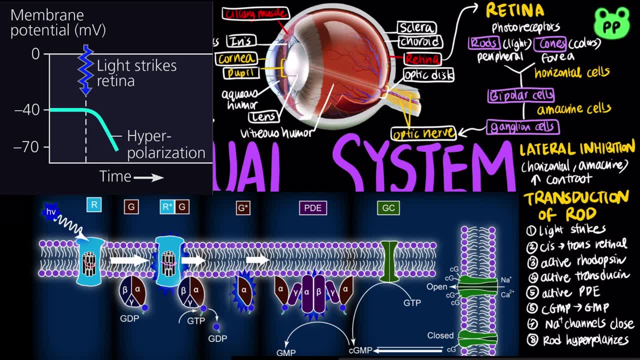 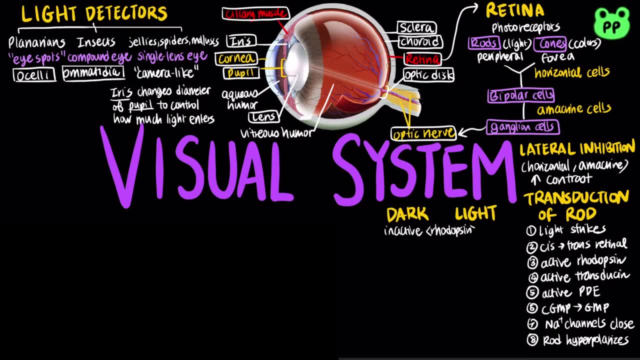 leading to the closing of sodium channels and a decrease in the membrane's permeability to sodium ions. The rod cell hyperpolarizes. Notice that this is opposite of neurons, which depolarizes in response to action potential In the dark. rhodopsin is inactive and sodium 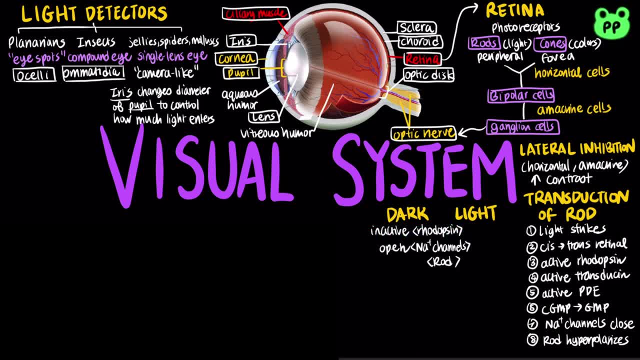 channels are open, The rods are depolarized, which releases gluamate to the bipolar cell. The bipolar cell will either depolarize or hyperpolarize depending on the gluamate receptors In the light. rhodopsin is active, which closes sodium channels, hyperpolarizing the rods. 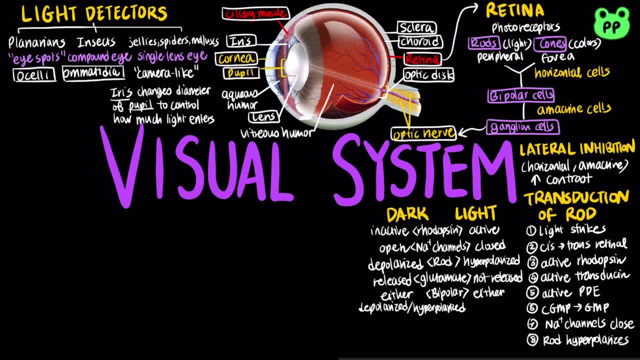 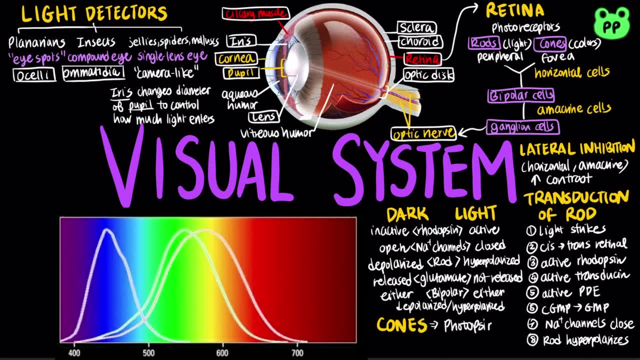 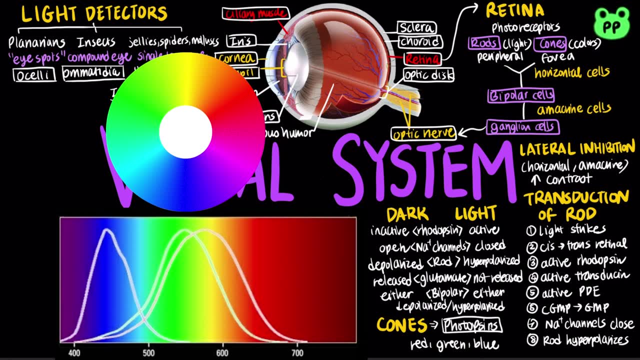 and, as a result, no gluamate is released, while bipolar cells could be either hyperpolarized or depolarized. The cones contain three pigments called photopsins that detect light of different wavelengths- red, green or blue. Essentially, all the colors we see are encoded by these three. 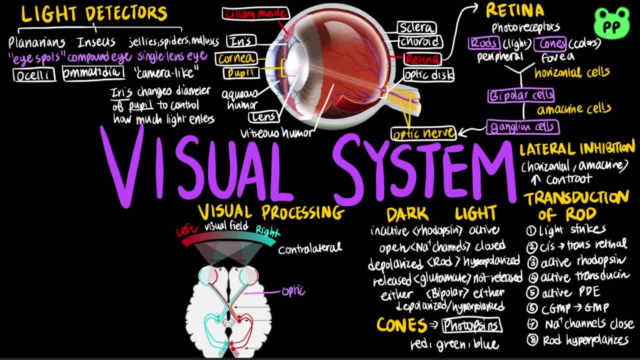 photopsins. The optic nerves transmit sensations from the eyes to the brain. Two optic nerves meet at the optic chiasm near the center of the base of the cerebral cortex. Our brains process visual information contralaterally, which means that sensations from the right visual field are transmitted to the left side of the brain, whereas sensations 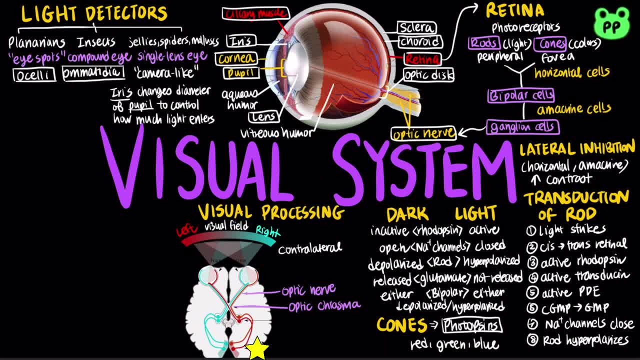 from the left visual field are transmitted to the right side of the brain. Note that each visual field, whether right or left, involves input from both eyes. So it's not like the right brain receives information from the left eye. It's from the left eye, So it's not like the right brain receives. 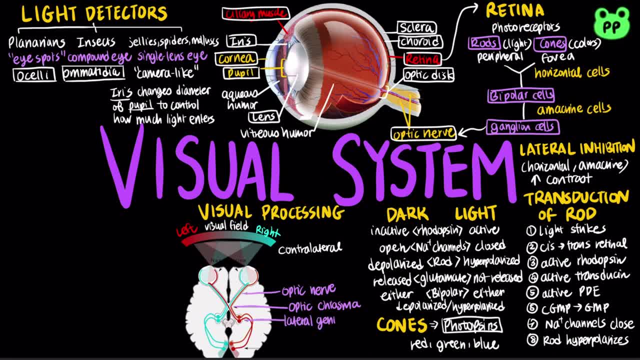 the left visual field of both eyes. Within the brain, most ganglion cell axons lead to the lateral geniculate nuclei, which relay sensations to the primary visual cortex, one of many brain centers that cooperate in constructing artificial perceptions. The human eye focuses light by 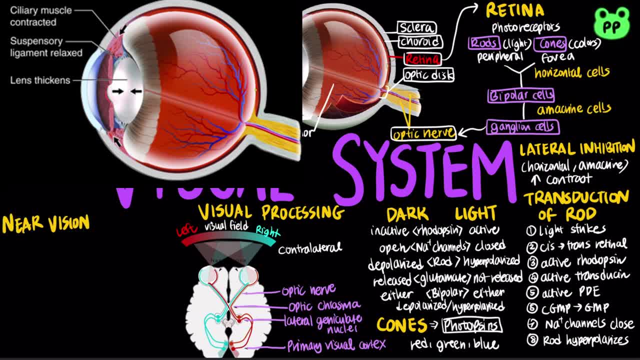 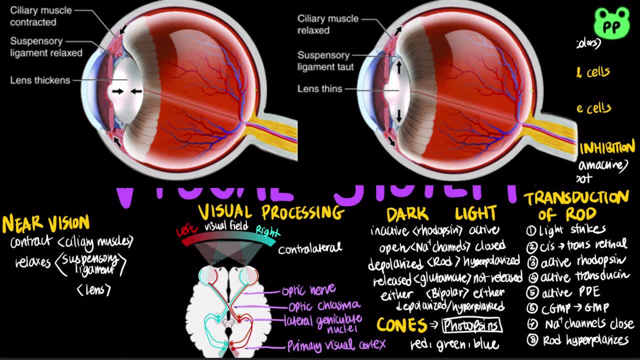 changing the shape of the lens: To see near objects, the ciliary muscles contract, relaxing the suspensory ligaments, which makes the lens thicker and rounder. To focus on distant objects, the ciliary muscles relax and the suspensory ligaments pull against. 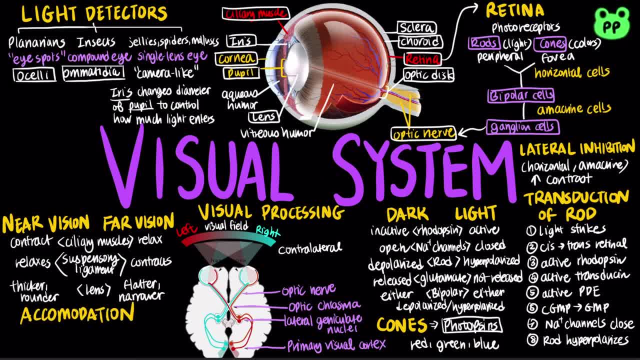 the lens making it flatter. The term accommodation refers to the change of focus from distance to near objects.